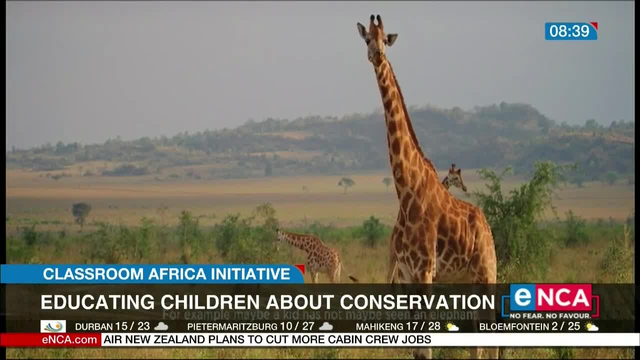 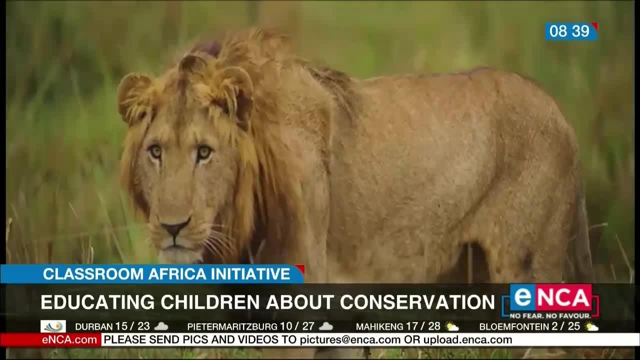 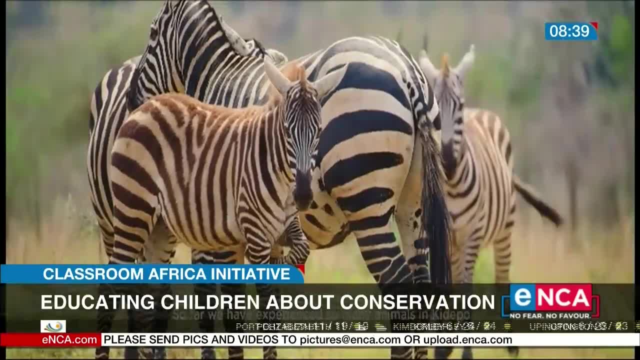 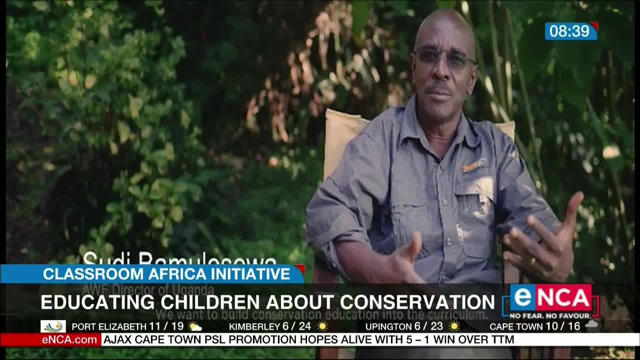 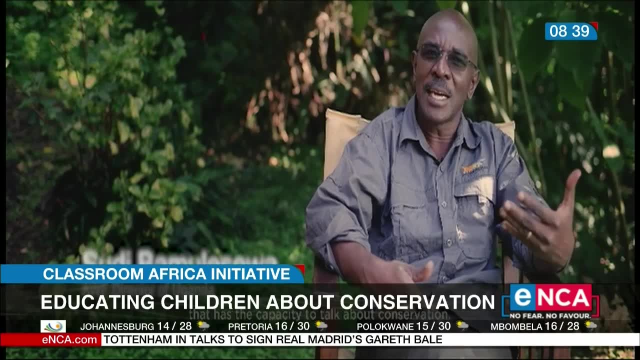 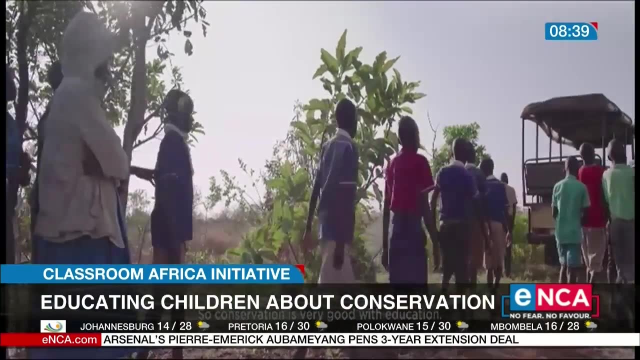 Again, for us, we believe that there's a direct correlation between illiteracy or lack of an education and wildlife crime or communities, but participation in illegal wildlife trade. And for us in the African Wildlife Foundation, we believe that access to a quality education by the communities provides an 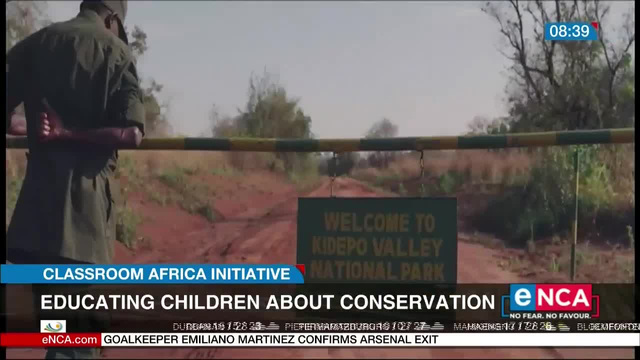 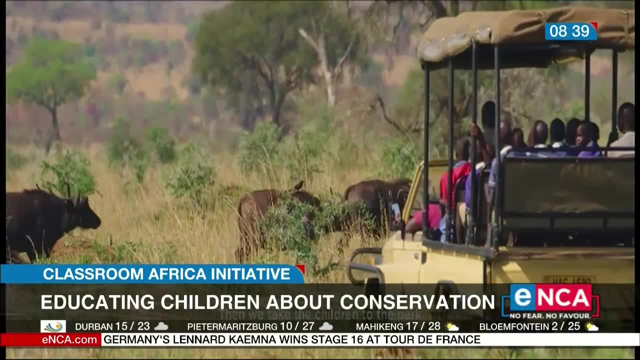 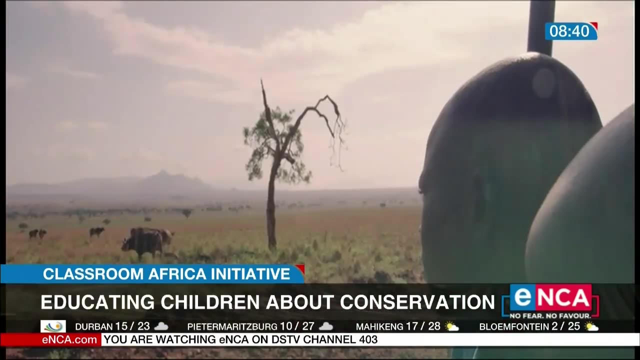 alternative, sustainable livelihood solution to help fight this crime. Tell us what is lacking at the moment, what hasn't been achieved up until now and why this is only really happening now. Well, obviously, for obvious reasons, where we do have the landscapes. 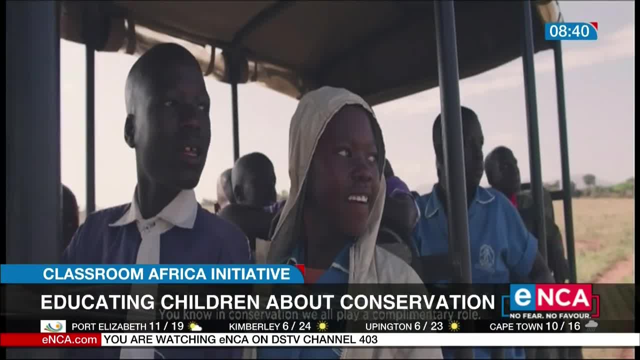 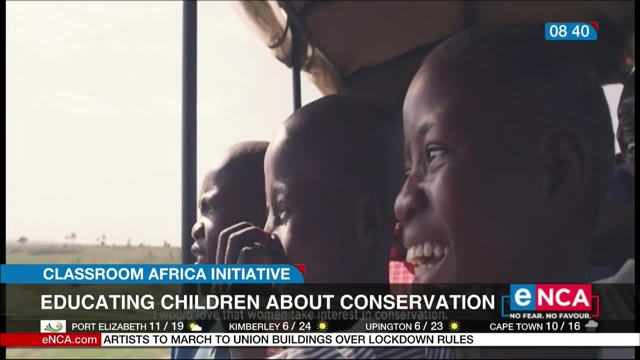 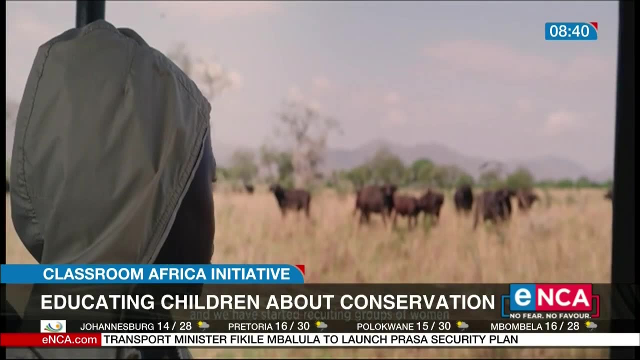 where we do have wildlife across Africa, areas in which the communities that live in are most marginalized communities in which children have the worst education indicators. So for us, this does matter right now, because we believe that if we're able to support education for these children, 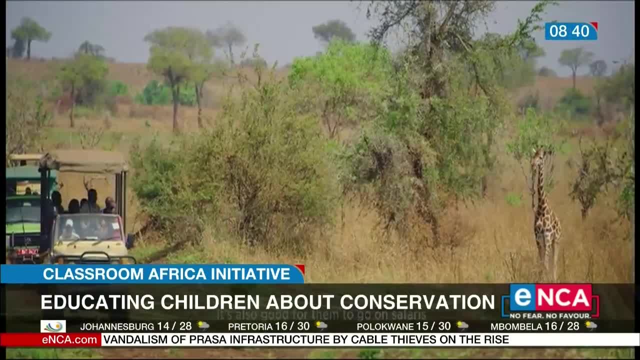 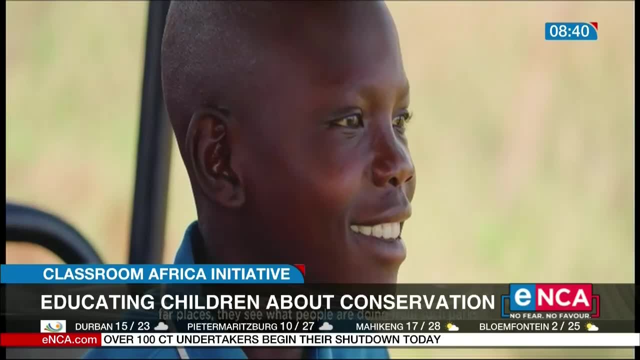 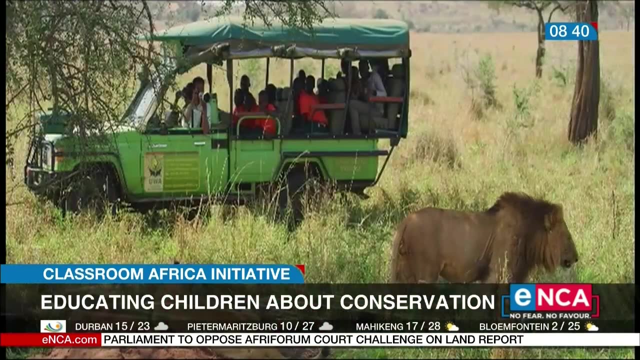 we're able to inspire future leaders, we're able to bring in a shift in the mindset towards conservation, And what is lacking right now is a push, obviously across the globe, And what we are advocating for is the donor communities, the international community, to be able to support conservation efforts. 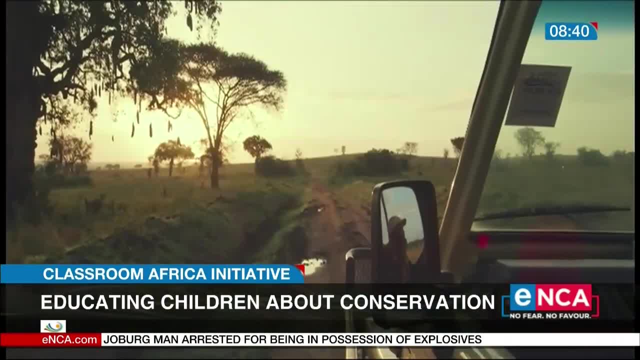 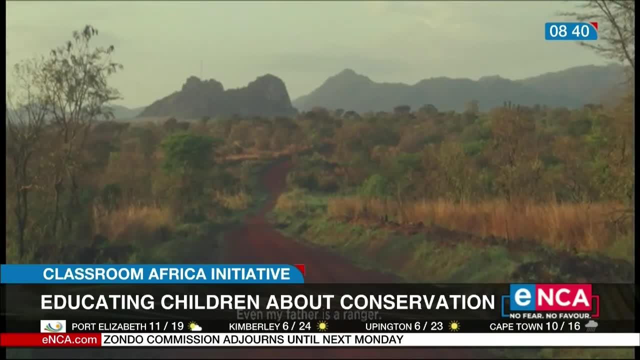 That includes conservation education programs that we have in AWF, anti-poaching efforts that we have, and so on and so forth, And working closely with our communities, our governments, will be very, very key for us to ensure that we achieve this. 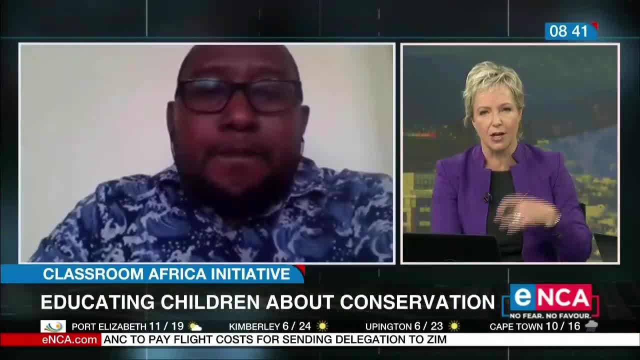 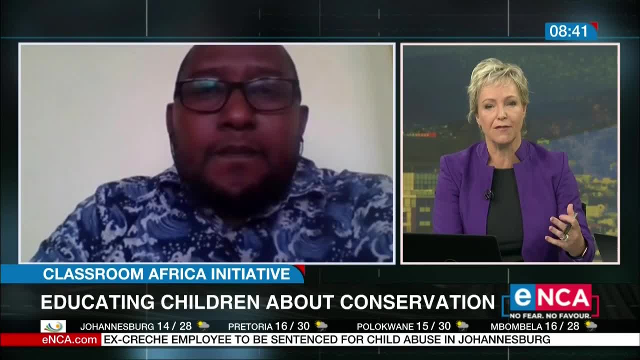 It's very important, isn't it bringing the community in? You say that so many of them have been marginalized for years, and especially when it comes to fighting off the poachers. You've got to give them an alternative, You've got to give them a buy-in. 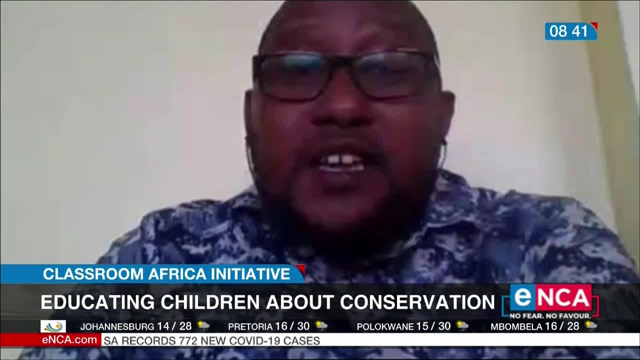 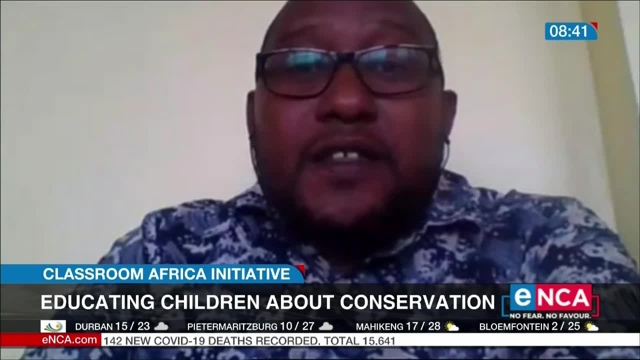 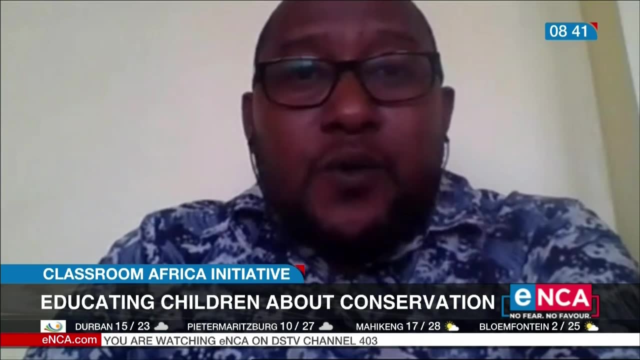 Yeah, most definitely yeah, And essentially, if you're able to have the ownership of these communities, to be able to change their sources of livelihoods that are not sustainable, that are not environmentally friendly, this is the way to go, And children are the best way to do this. 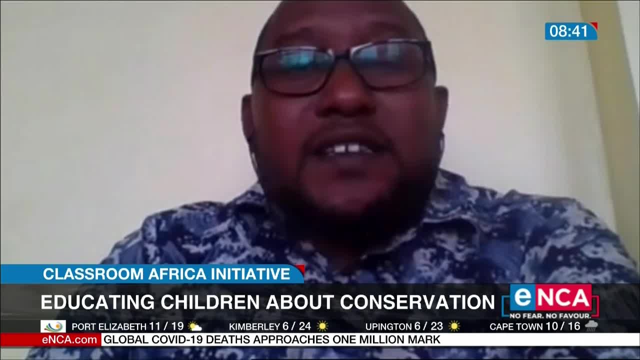 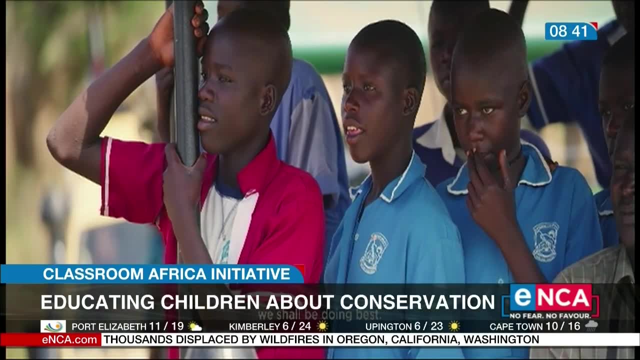 If you're able to have them access an education, then what we're saying is that we will be able to have a lot of changes. For instance, we're having an impact story in Uganda, in the Murchison landscape, where we have a girl that was not able to access an education. 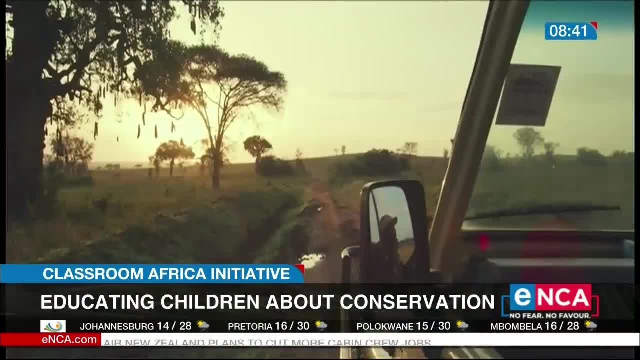 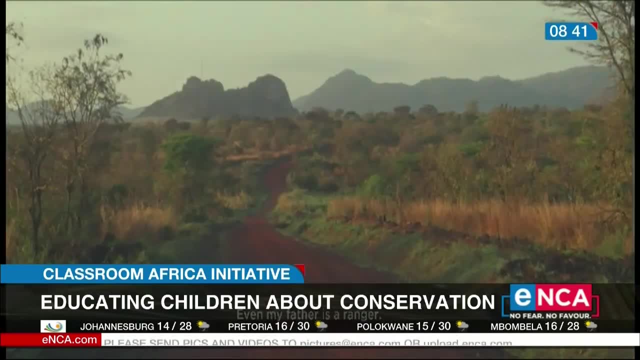 but through support from AWF and its donors, the girl who was to drop out of school now, at 17 years, is in secondary school at the first level, And this is a person who is a champion in conservation, So we're seeing that in the future. 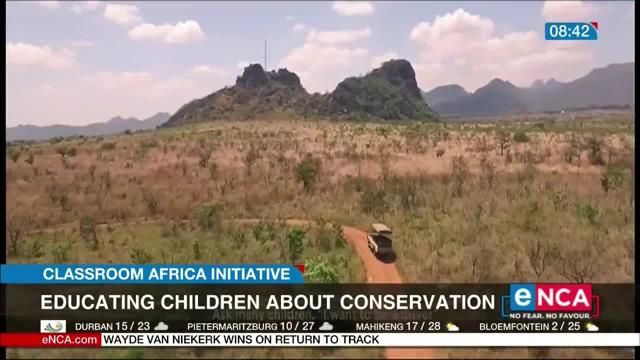 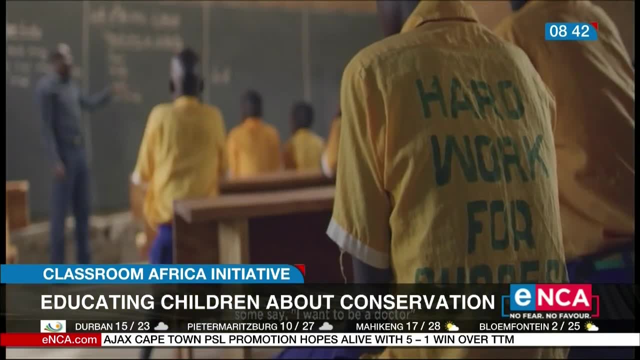 these are the people that rely on to ensure that the wildlife and our wildlands in Africa are protected. And I mean, you see, as you talk, we're looking at quite incredible pictures of the children studying, but also of what we have on this African continent. 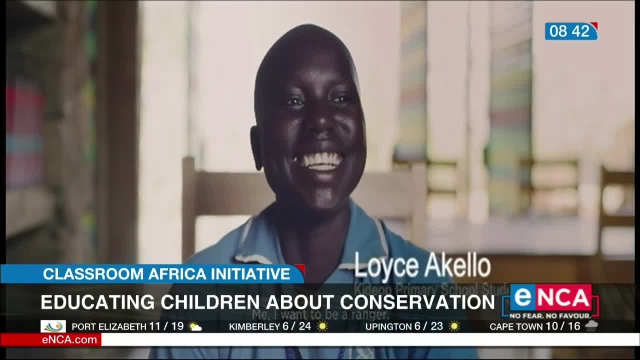 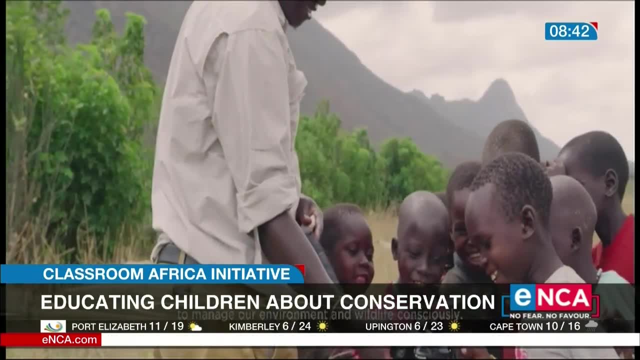 And it really is something to be proud of, isn't it, Particularly at this time. I mean, this is something that could just generate if we tackle it properly. it's something that can generate so many jobs, such a sustainable future for so many people. 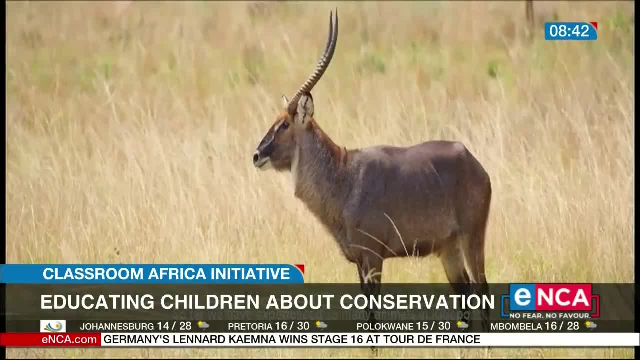 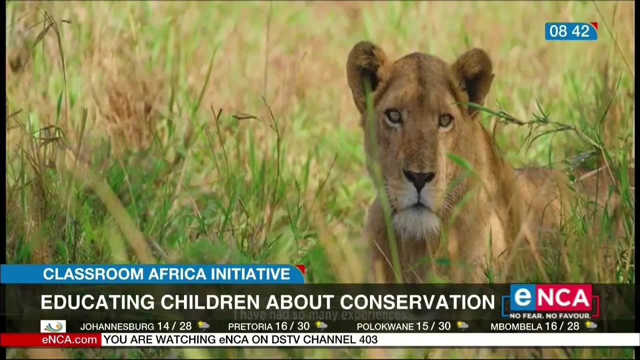 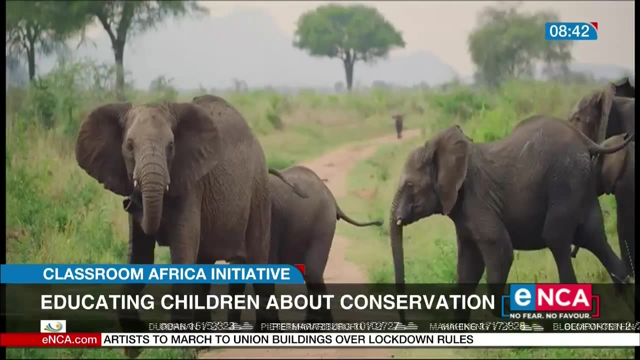 Indeed, Jane. that's incredibly correct. The fact that this provides an alternative livelihood solution for them, for their families and for the children basically changes a lot, And when you look at the videos that you're talking about, you can see the Kidepo school in Uganda that is being aired. 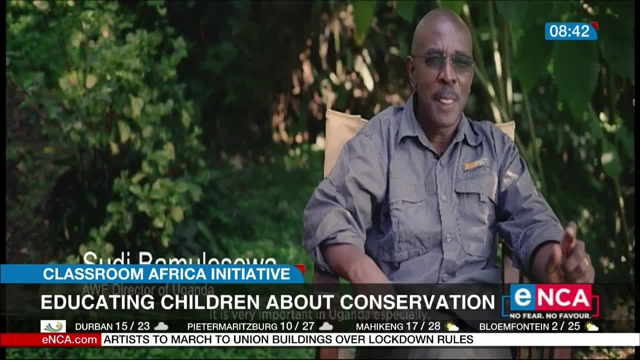 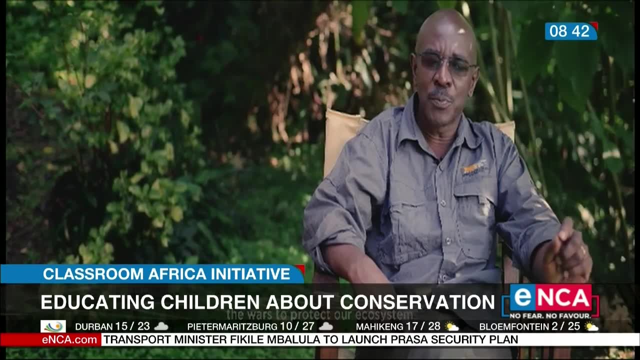 You can see that is a place from a school in a very remote place in Uganda, But you can see that the kids in the school are able to access wild class education just like other kids across Uganda and across the globe, And the fact that this is something 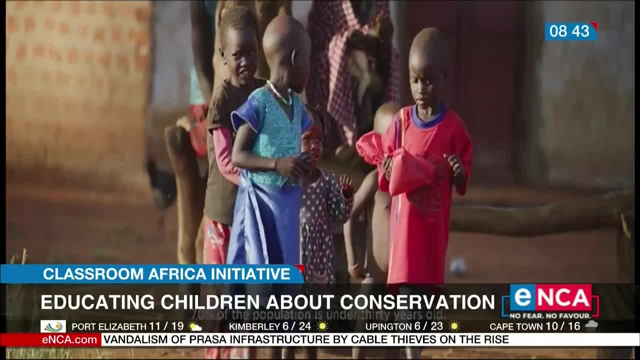 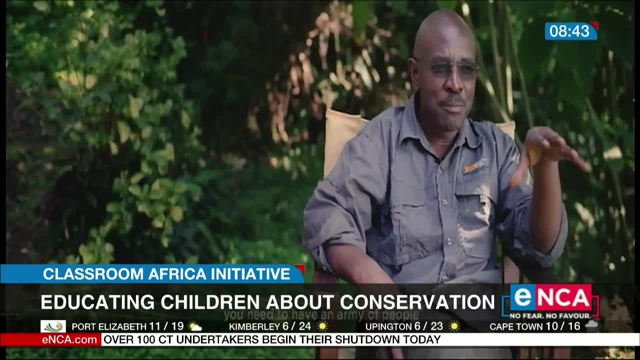 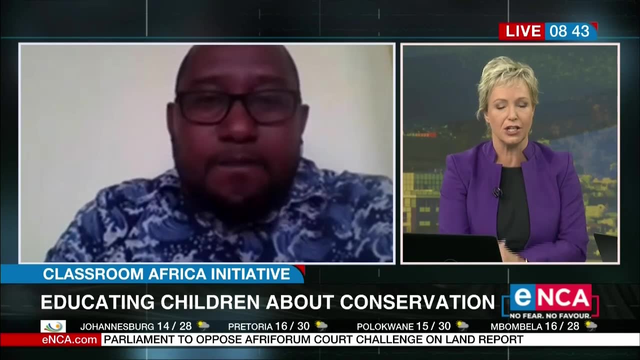 I mean, education is a dream to some people in such places, but making it a reality is such an incredible thing that we value at AWF, And is having access to technology a challenge here? Is this something that needs to be addressed in order to keep this initiative going?